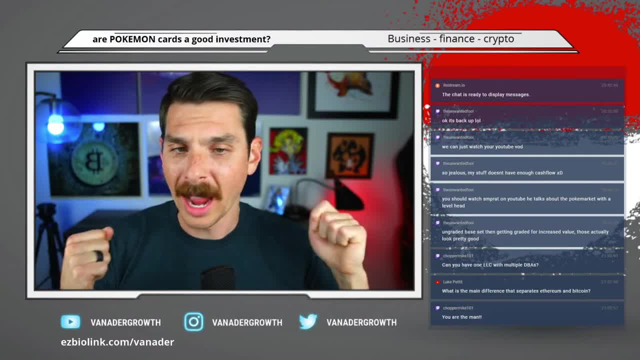 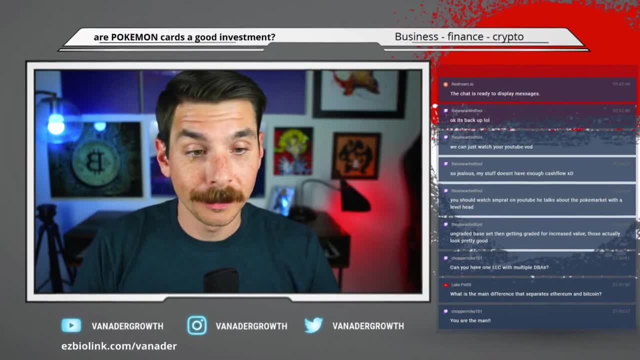 for me to lease a Corvette for the for our business, for me to for advertising and marketing, but you're still driving around. uh, you know, a base model Tesla costs way less. You're still. it doesn't matter, Even if there's disparities within the company, the money that comes out. 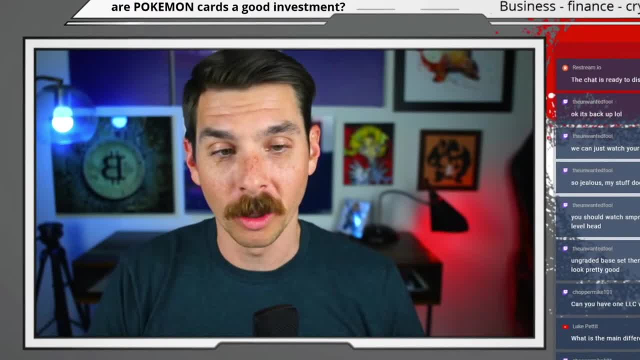 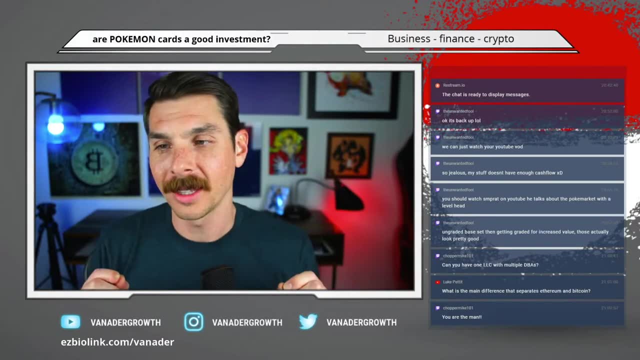 still has to be pro rata. So I'm pretty sure you don't want to pay for my Corvette. So that's why I don't recommend having more than one person in an S-Corp, because there's little things like that that make it difficult to be flexible. Here's the solution You form. 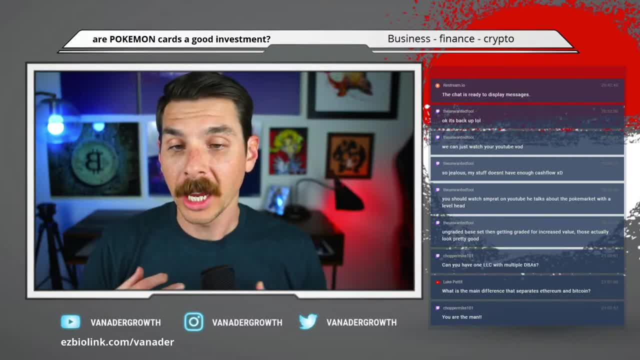 an S-Corp with more than one person in an S-Corp. You don't want to have more than one person in an LLC taxed as an S-Corp- Just you. That is now your holding company. That's now your baby. 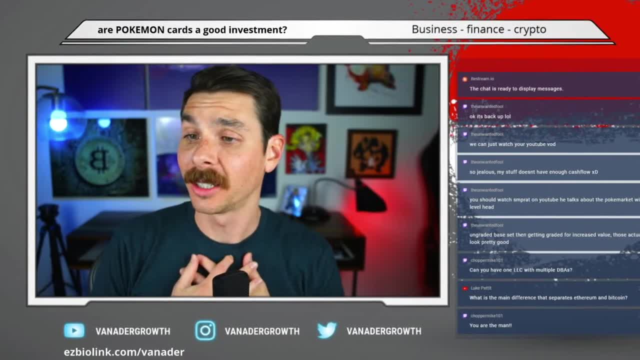 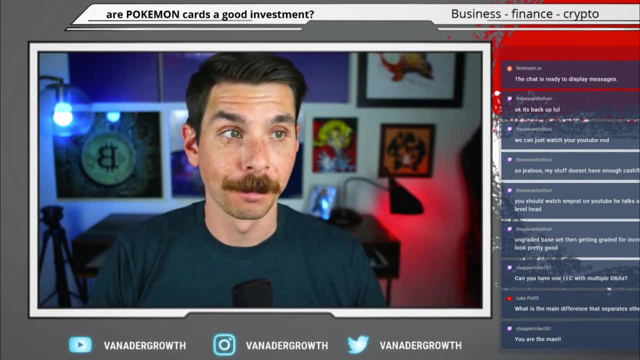 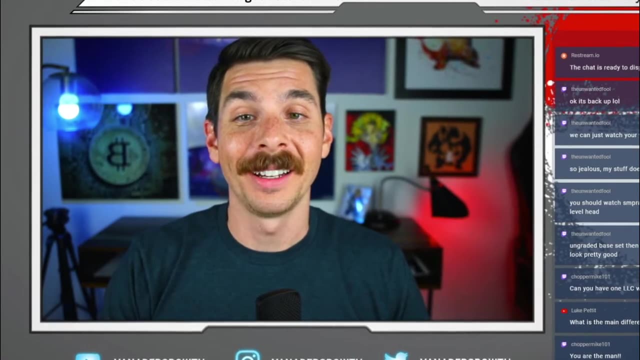 That's your company, that's going to be with you forever And that's the company that's going to do business with other companies. So the next time you want to form an LLC with somebody and try out a business idea, you form the LLC, but instead of you the owner being on the paperwork, you have it. 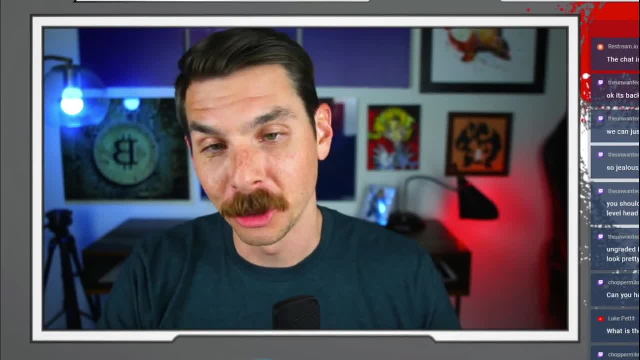 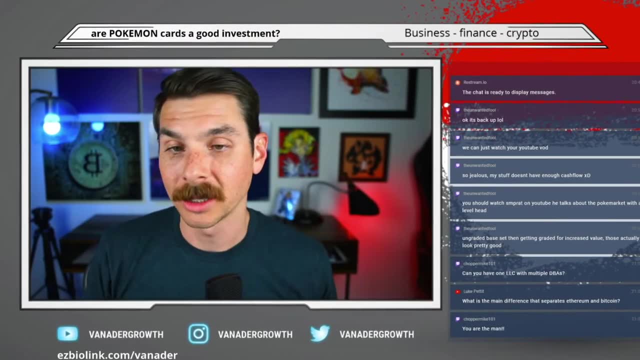 you have your holding company on the new LLC with your new business partner. You'll have your S-Corp and then your business partner and you'll both own the LLC and it will be taxed as a partnership. This way you don't have to deal with the pro rata distribution rule and you guys can do. 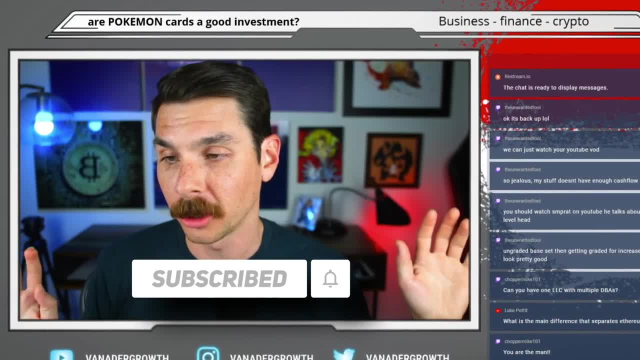 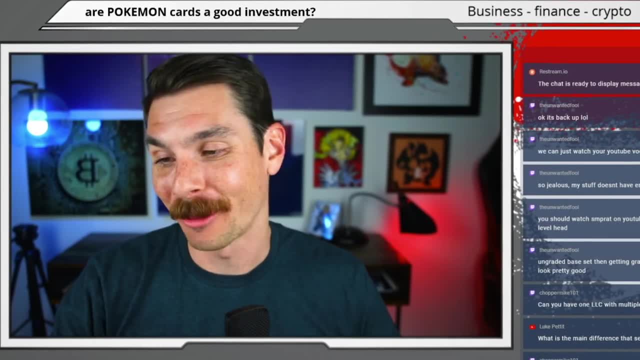 whatever the fuck you want, whatever the hell you want, When you have an LLC taxed as a partnership, you can do whatever you want, right? I think that's pretty cool. It's a cool way to go about. I hope that answered your question. man, I get on these soapboxes and I ramble. I'm sorry. but I hope it helped. 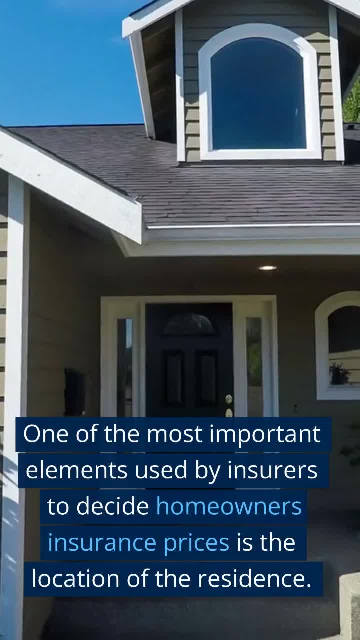 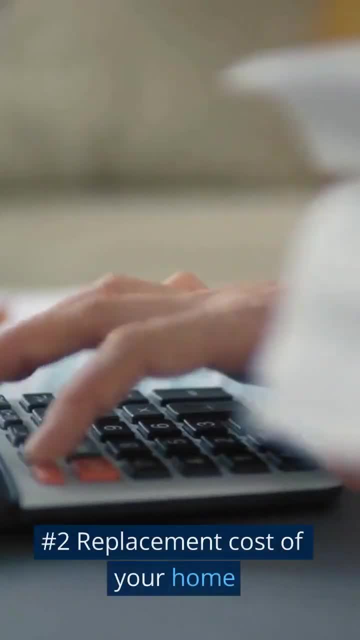 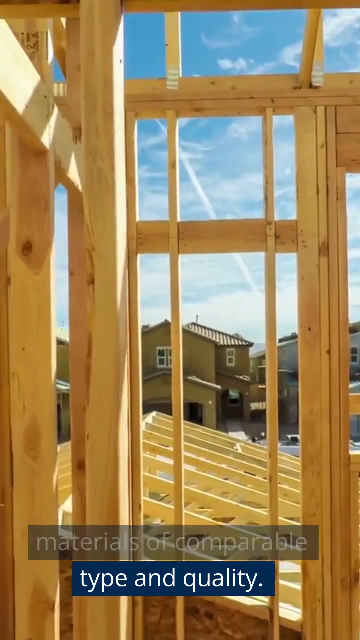 Number 1. Your home's location. One of the most important elements used by insurers to decide homeowners' insurance prices is the location of the residence. Number 2. Replacement cost of your home: The cost of rebuilding your home using construction materials of comparable type and.